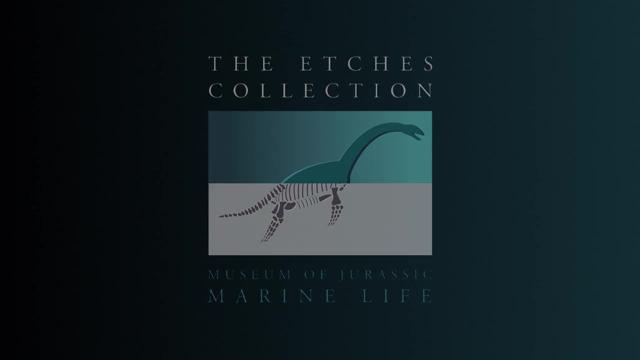 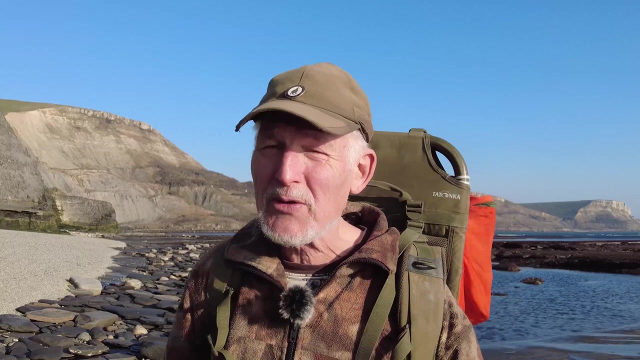 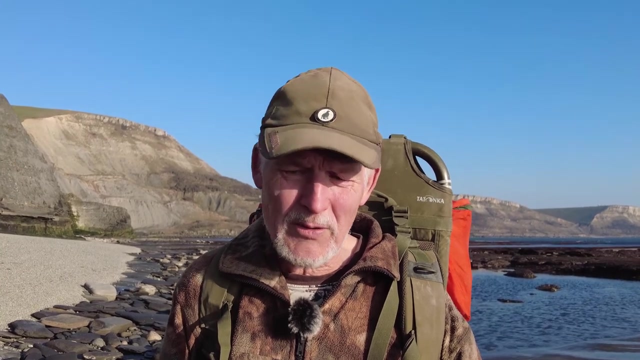 Well, you drift into it in some ways. You become a hobbyist and collect fossils, like I've done, and then go from there. If you really want to be a paleontologist, then if you want to do the university route, you've got to go to university to get a degree, get. 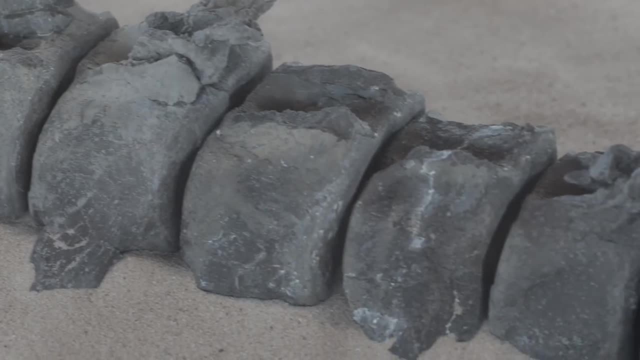 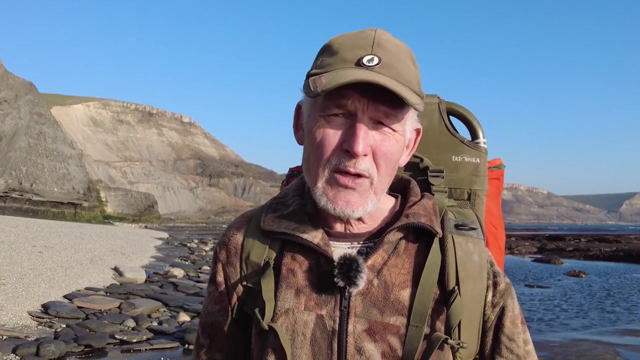 a PhD in certain parts of paleontology, but vertebrate paleontology, which is everyone wants to get into, that, is a very close shop. There's not many jobs going in universities and museums to be a full-time paleontologist, certainly in this country- America, China. 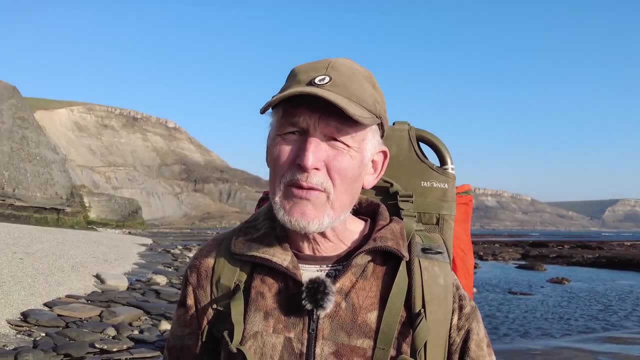 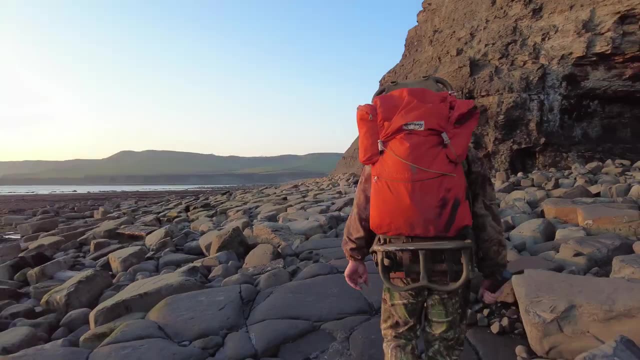 yeah, they're crying out for people, but in this country no. So it's more. I would suggest to anyone who wants to be a paleontologist, then do it as an interest and a hobby first off, before you really want to get into doing it as a job. There's not a lot of money in. 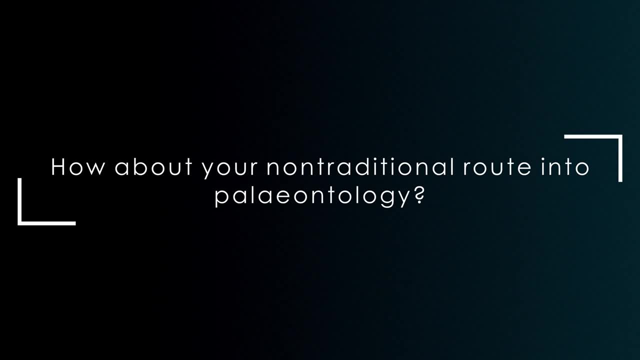 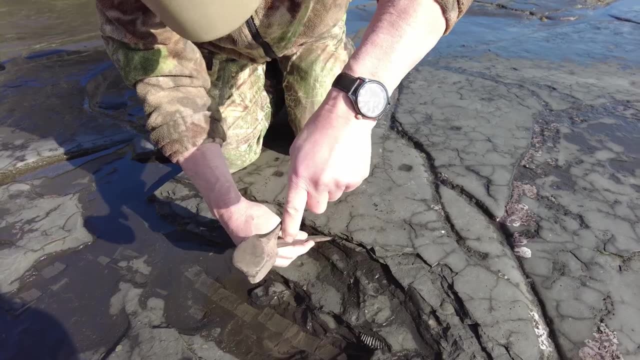 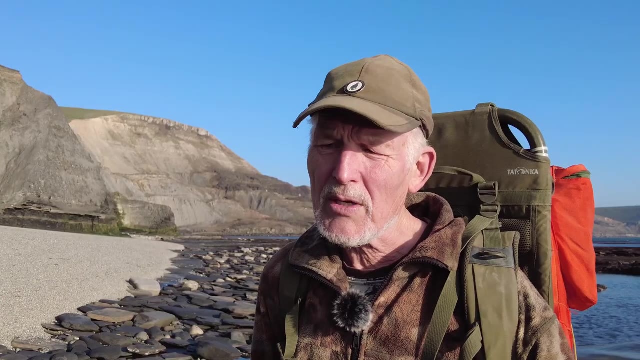 it. I can guarantee you that Non-traditional route. Yeah, that's interesting because what I did, to be pretty frank and honest, if you collect fossils, like I do, from a specific locality, you've also got to know the geology. So what I used to do is to go onto the Bristol University extramural courses. 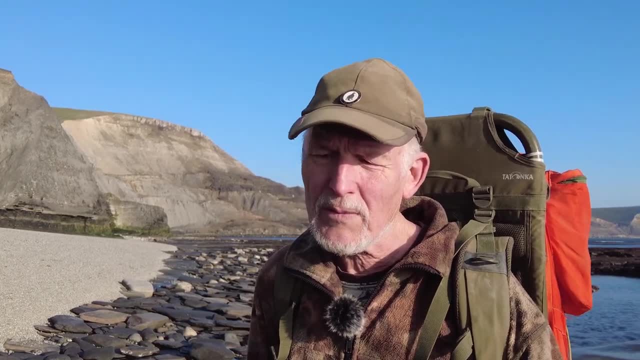 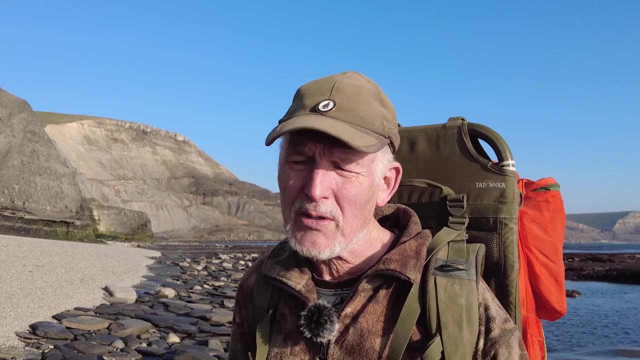 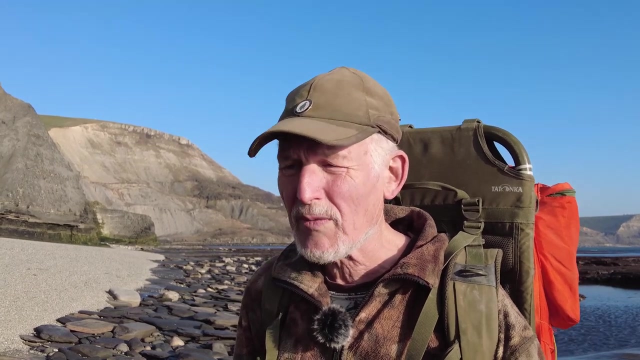 So they used to do courses outside of the university for interested parties and it may be over a weekend or three or four days and you would learn about geology in certain areas and goodness knows what. I then used to go on Dorset County Museum used to do evening talks on specific subjects. 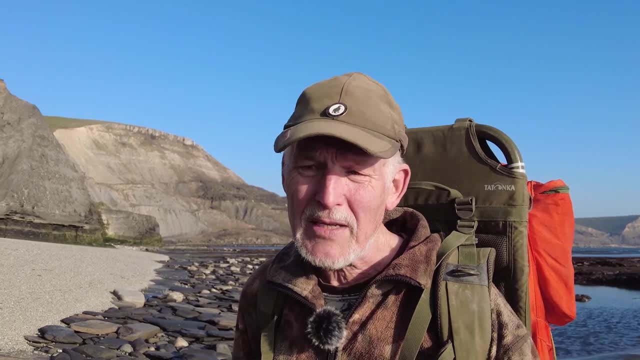 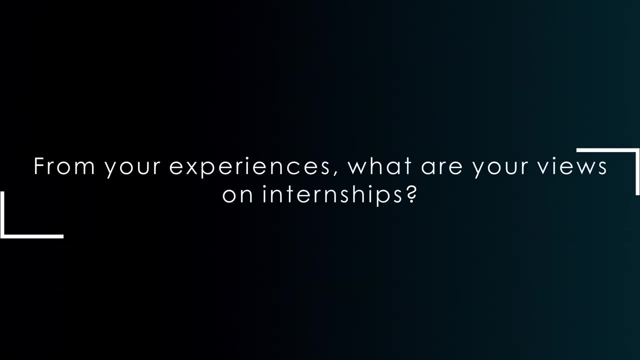 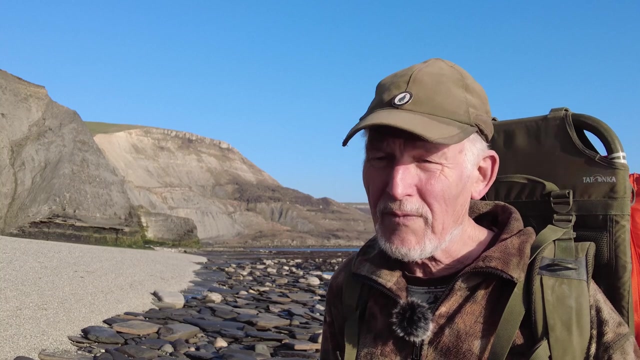 related to geology and that's really then getting every available book on the subject and learning it from there. Oh, the interns we've had, right, so yeah, we've had interns in the museum. They're doing this part of their outreach from the universities on certain things, These students we've had. 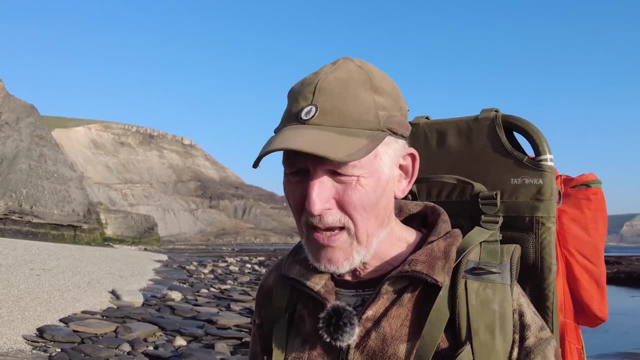 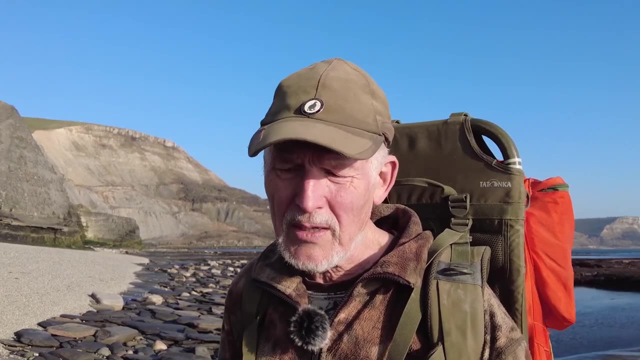 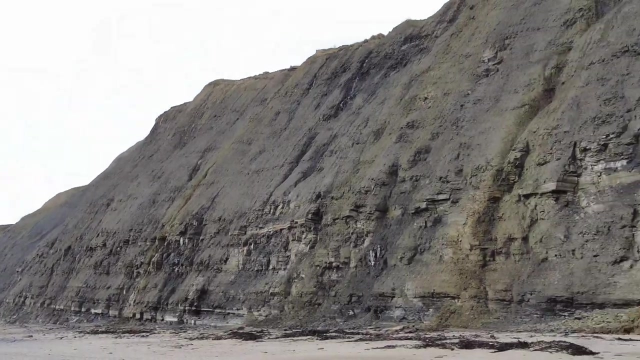 have been bloody good. to be pretty frank and honest, they were certainly interested. they come up with a lot of ideas, certain aspects of the museum, like one of them did a display showing a sort of section of a cliff, showing the alternate mud, stones and shells and everything else. that's really, really good. she also, which was brilliant- 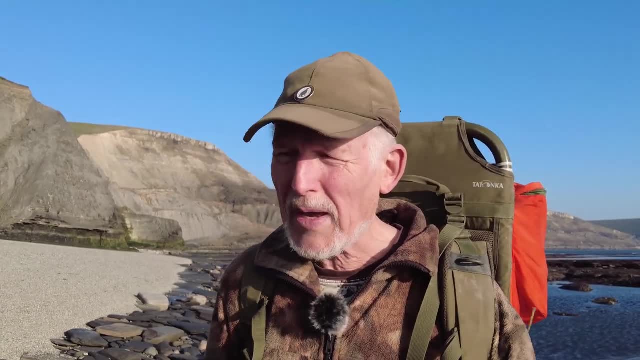 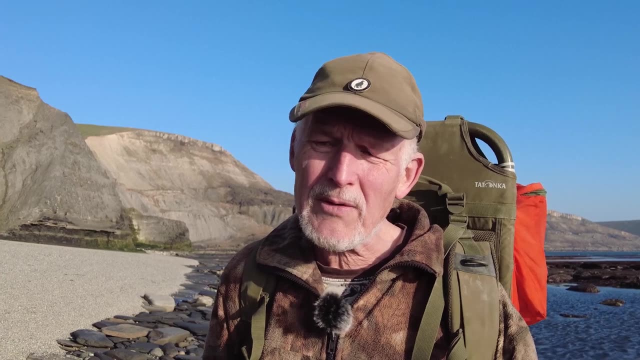 telling she was really artistic. she had a map of Purbeck with a sort of pterosaur imprinted over it and it looked really really good. so the interns, yeah, been good and they're. they're sort of what they want to do later on in life. I don't think they're sure of themselves. they want to do a. 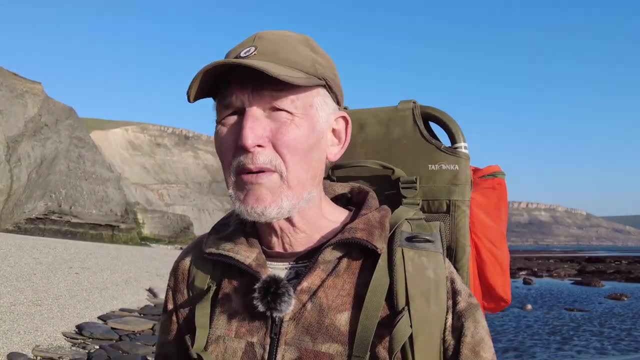 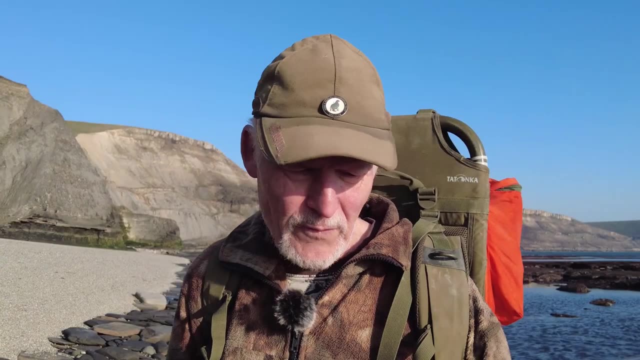 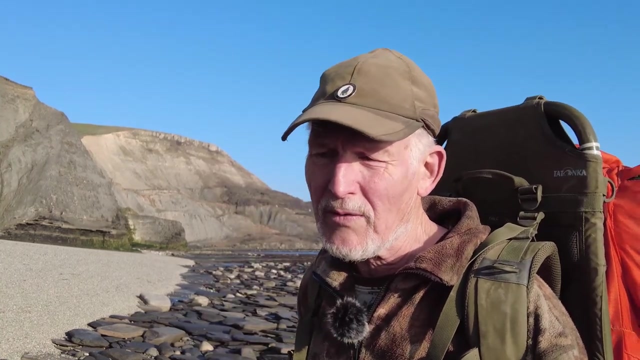 degree, get a degree and then decide which- where they're going to go for their future after that. whatever we can do for people will do it. if there's anything that they if they want to become as a volunteer or we do. now we've got a lovely girl from Southampton University that 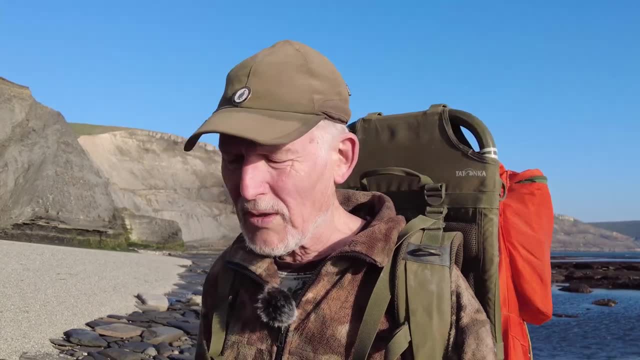 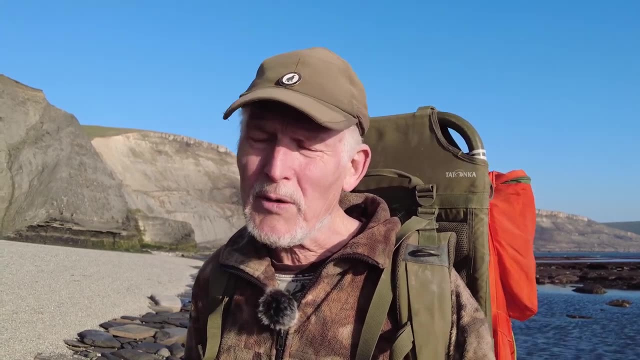 unfortunately, she well, she can't come here at the moment because of the shutdown, but she's really good, she's come there as a volunteer and she- she actually is. it for her is to put down as an experience to work in a museum. that a lot of 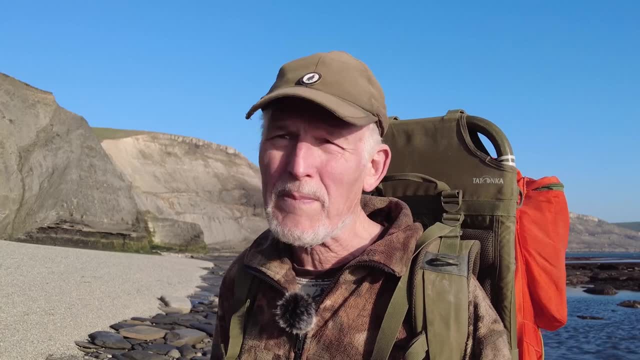 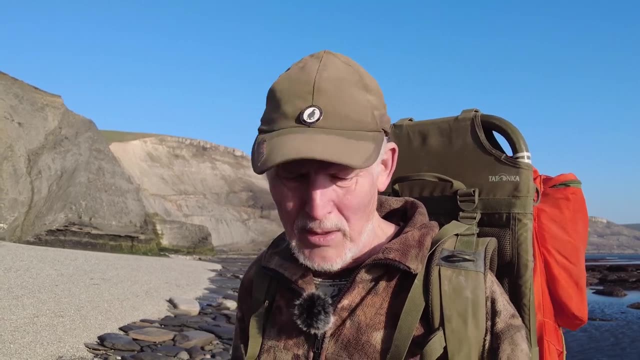 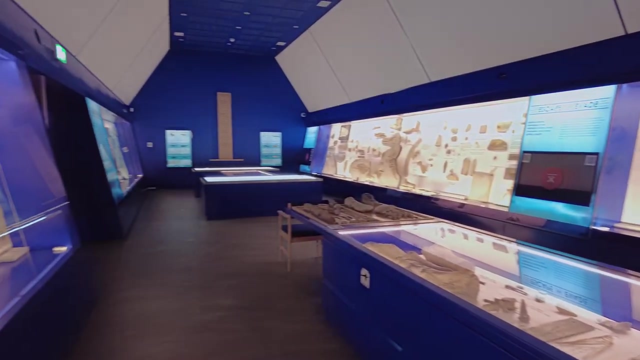 people won't get. so she's come as a sort of volunteer or we pay her just as expenses and from that she gets a good grounding in in what she wants to do in, in other words, the run in the museum and looking at the fossils, following up that sort of particular you know aspect as well. so it's. 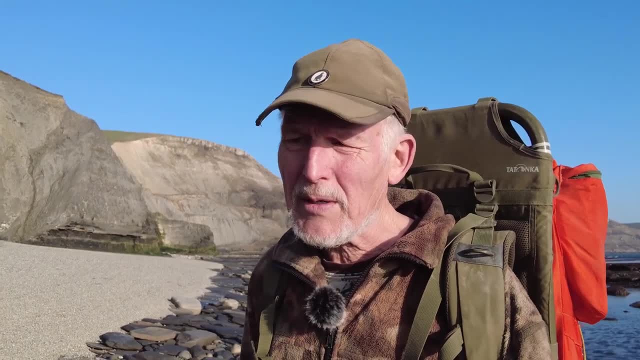 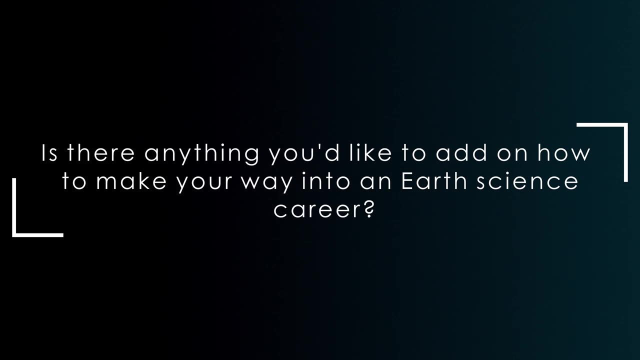 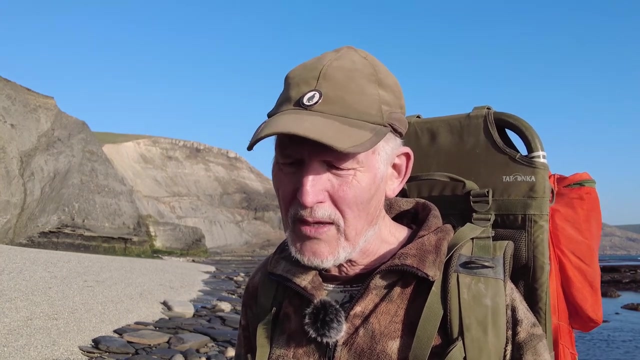 a process for courses. they, yeah, they, they love coming and working there and, from for their perspective, they they get a grounding in working in a museum. I would say to anyone who's following that sort of course, if you, whatever you do with it is, actually have a very open mind. don't close your mind to certain things. in other words, 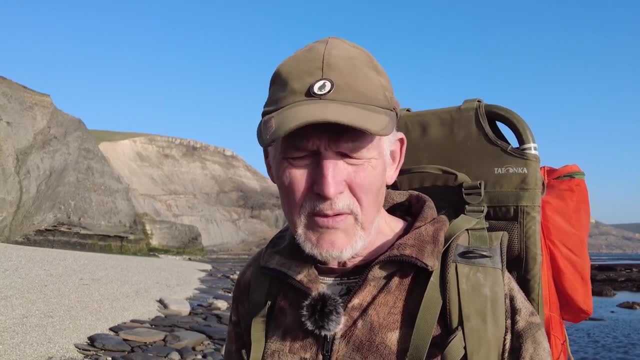 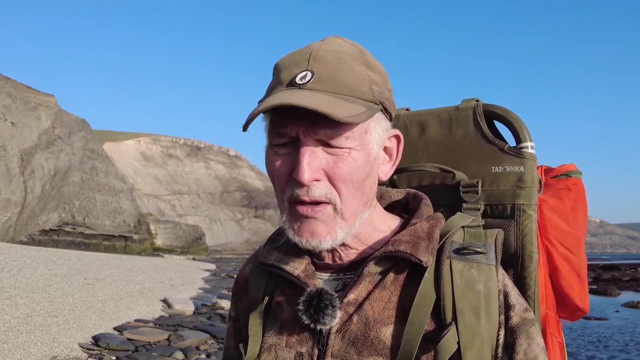 if you're doing a course and some professor comes up with something that you really you know not sure of or don't accept it fully, find out for your own self. so be inquisitive. look, do more than the. the people are going to make their way in life. in paleontology is the people. they're not going to sit on their. 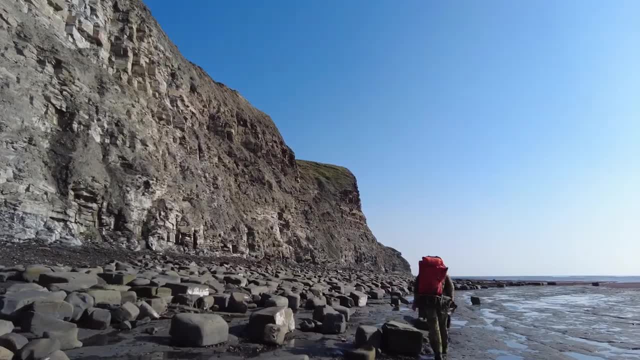 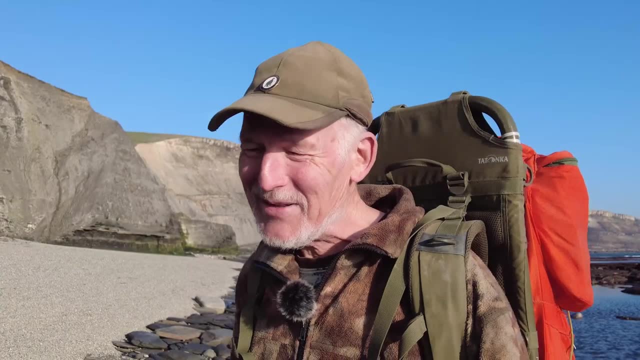 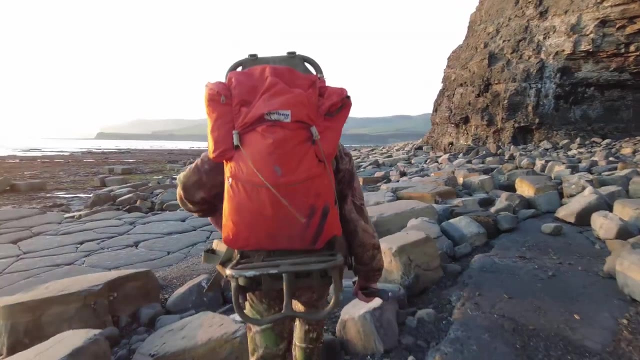 bums and just do the minimum. you really got to get out there and you've got to be passionate about it. that's a that's an easy question. I mean, okay, coming from a plumbing background, you get all the stress and worry. now I'm working, I'm out in the field, I collect as and when I can.